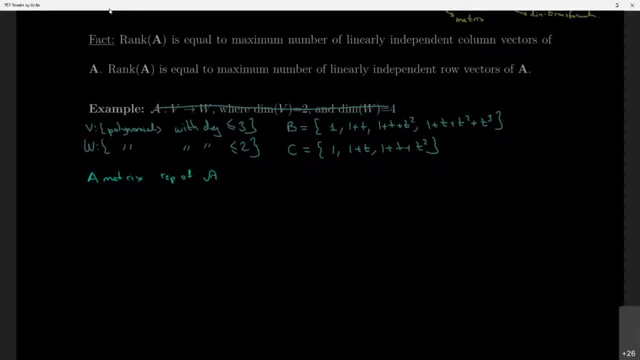 Matrix representation of a linear transformation. let's say A. And when I say the matrix representation, what is the first question to ask? With respect to which basis sets right? So this is with respect to B in the domain and C in the codomain. okay, Maybe. 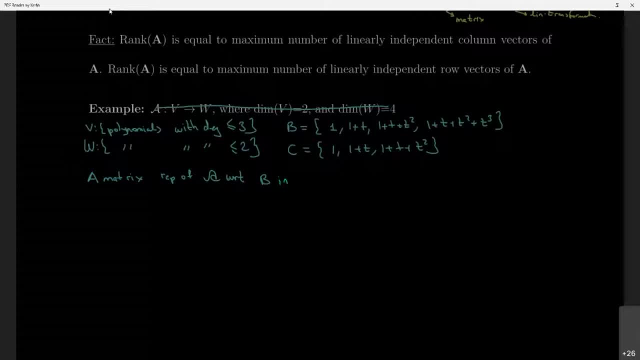 I can write explicitly: So B in with respect to B in the domain And C in the codomain. So I can write that A is like from B to C. okay, All right. this A matrix is given as follows: It's not going to be enough space, So A is equal to: let's. 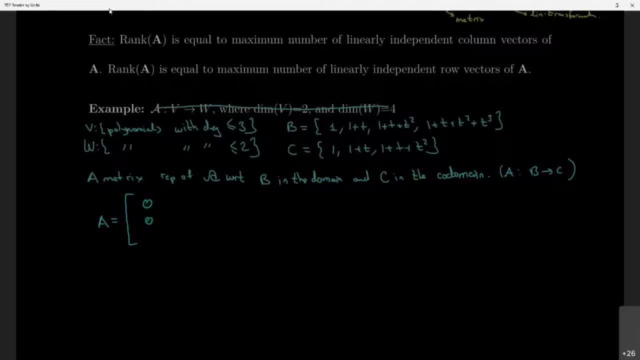 see what it is: 0, 0, 0.. 1, 0, 0.. I should tilt my arm a little bit. Minus 1, 2, 0.. Minus 1, 2, 0.. And minus 1, minus 1, and 3.. So yeah, 3.. All right, so the first question. 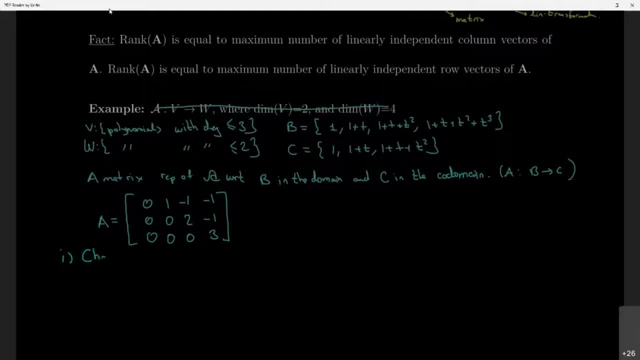 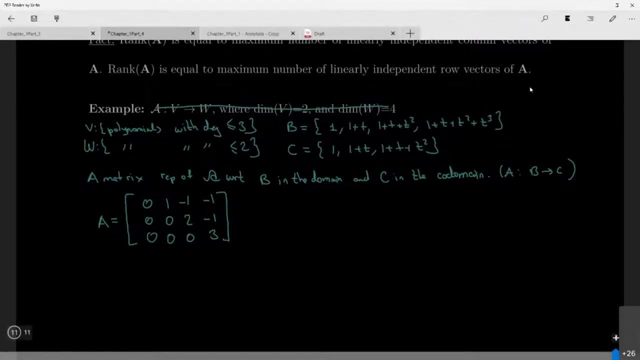 is So: change the basis in the domain as B bar. okay, And it is given as 1, sorry, this is not 1.. Can I redo that thing? Yeah, What was the shortcut for redo? What was the shortcut for undoing? 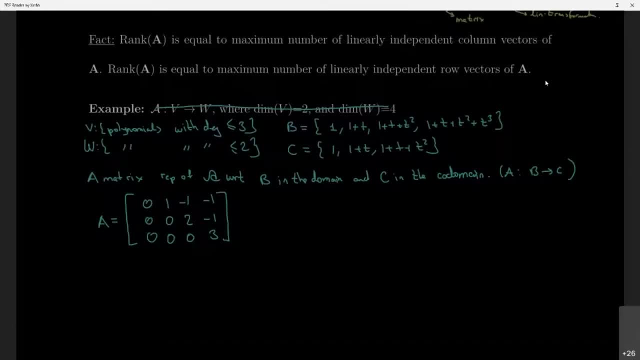 What was the shortcut for undoing? CTRL-Y, sir, CTRL-Y, CTRL-Y. Let's see, There is a teacher who enjoys simple things. I was very happy when I could bring it back Now. I was going to write 1.. That was the whole problem. 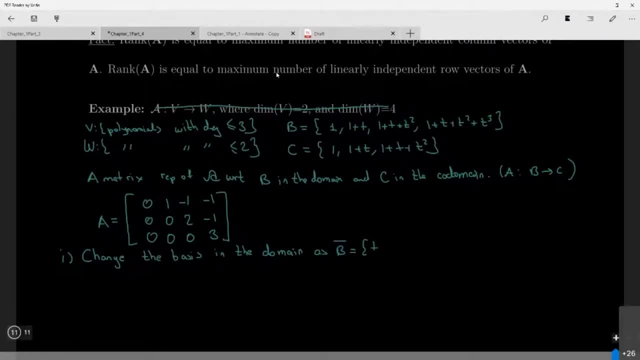 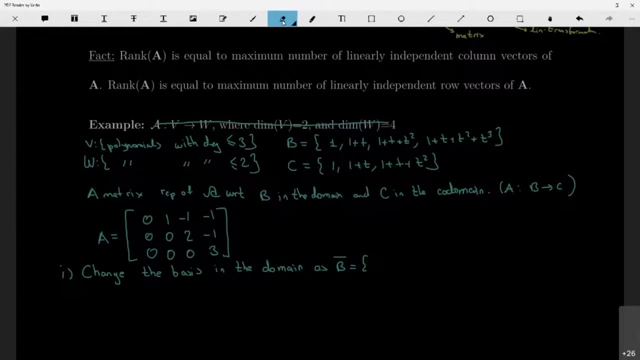 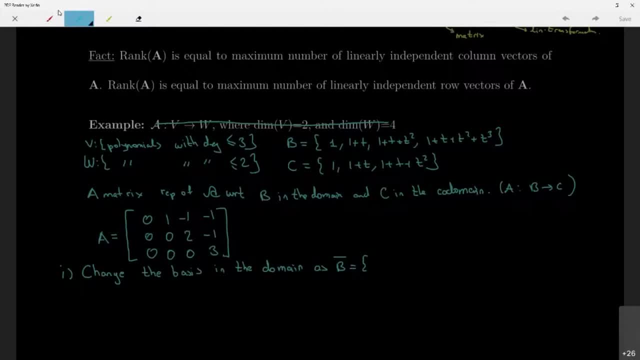 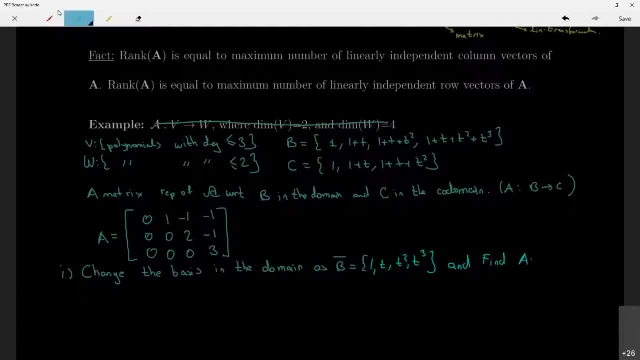 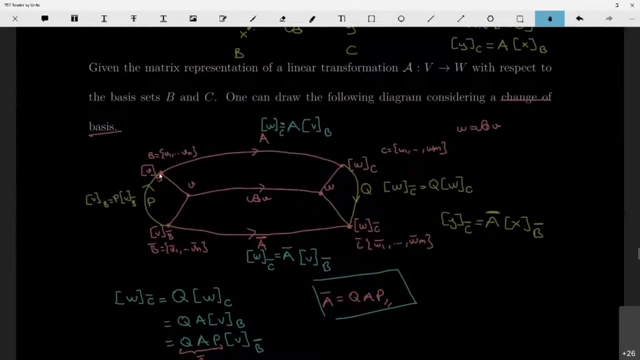 representation, let's say a1,, which is with respect to b bar and c. Okay, So how are we going to proceed with that? So if we go back a little, stop there, Alright. So this is our general picture, right? So I have this b basis and c matrix and this a representation, Okay, And if 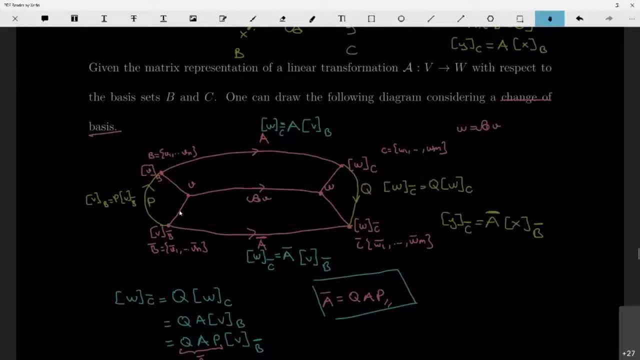 I would like to find this a bar in the sense that I only change b bar there, c bar and c the same, so q is almost identity. I can only say, if I need to only find this p matrix, and p matrix does this. it takes the presentation of the vectors with respect to b bar And 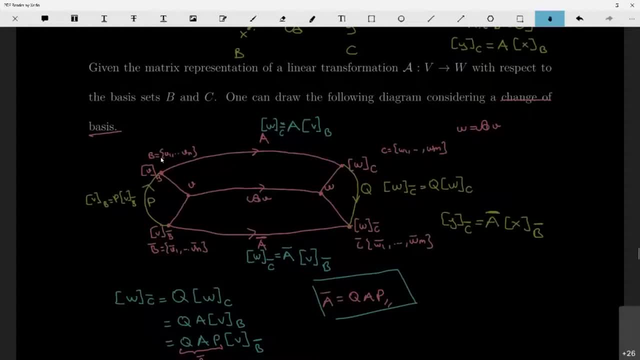 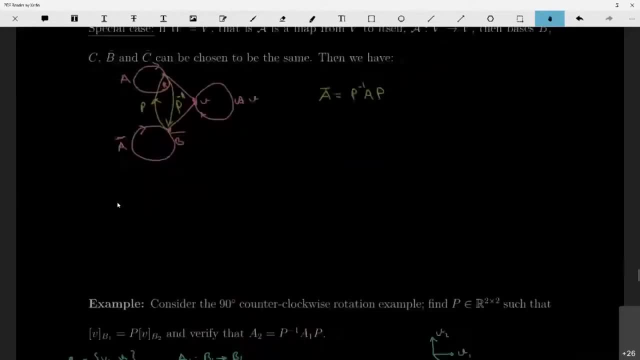 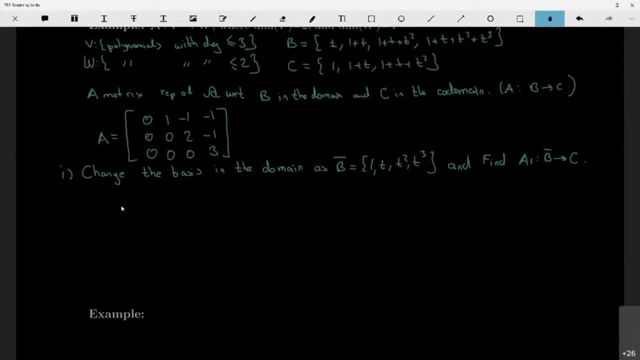 transforms them to representation of the same vector with respect to basis b by this matrix multiplication. Okay, So all I do the first step. I should find this guy, where is it? So I will have any vector v with respect to b. I should be able to write this p times: same vector with respect to. 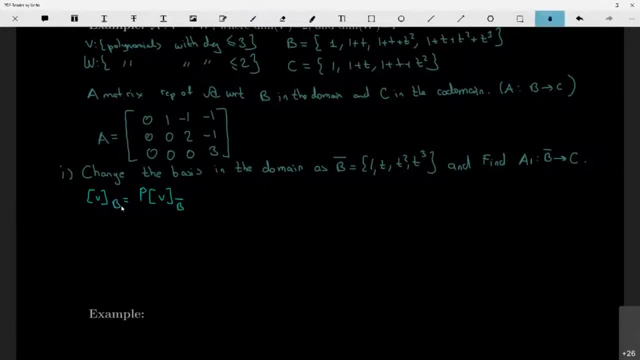 b bar. And how do you do that? And how do you do that? And how do you do that? How do you find that p matrix? Do you remember? Of course you remember, because you had a quiz last week, right? How do you do that? 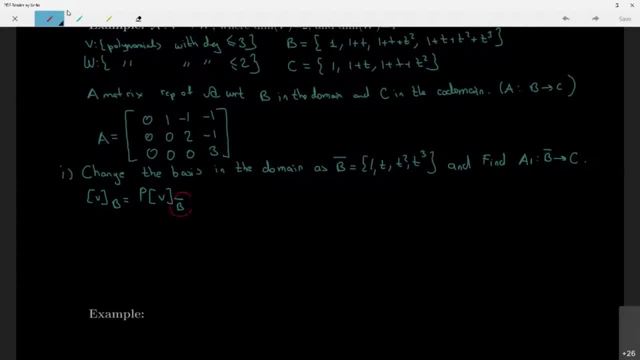 So if you write this, so write this basis vectors in terms of b, basis vectors, b the way saying b. Okay, Let's do that. In short, So let's do that. What is the? I write it directly. I say that you should now get used to it. 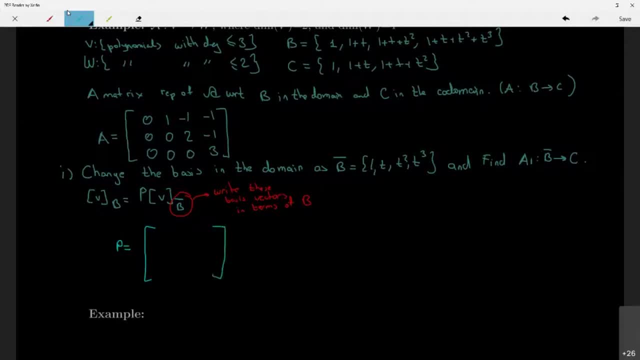 Let's write matrix directly together, okay? So let's try to write down the b bar in terms of these guys over here, right? So what is one equal to in terms of these guys? I mean linear combination of these guys. What are the coefficients? that corresponds to one. 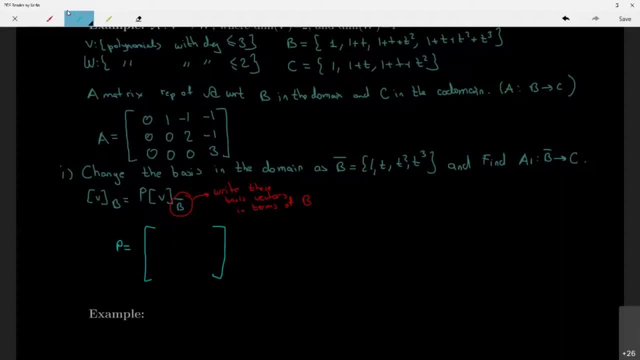 So X is the linear combination of these two guys, Exactly, and I write it here as the first column. How about t? t is equal to minus one one zero zero, zero. So this is minus one one zero zero. How about? maybe I can to show you. 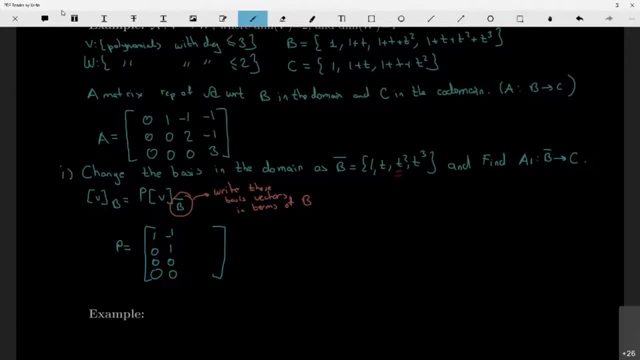 some color. How about t square? So t square is equal to this minus one zero, plus one zero, right? So if you subtract this guy, you get t square only. So I will simply delete those and write down the column immediately. It is zero minus one one zero. How about the? 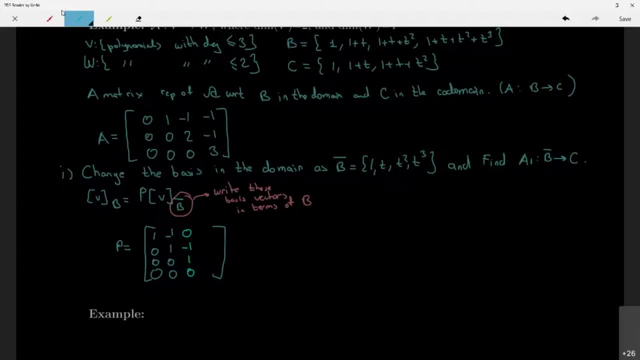 last column You tell me. I would like to explain it. I would like to express t cube instead of in terms of these basis vectors. What are the coefficients? Zero, zero minus one one, Exactly. So that's my p matrix. How about this? a one matrix, which is which was shown? 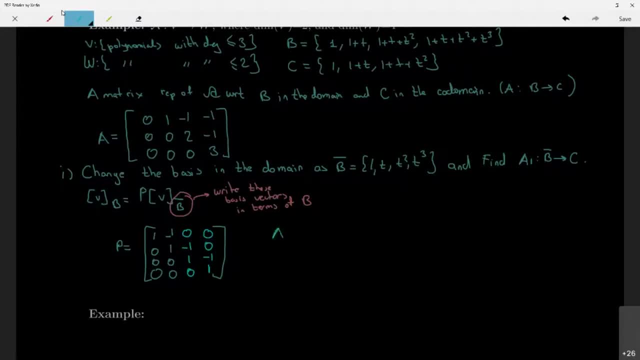 as a bar in the previous derivation. So what is a one? It is equal to a times p. OK, So I would get this pil matrix and multiply by this guy and apparently the result is this: 1, 0, 0 minus 2, 2, 0, and 0 and 3.. 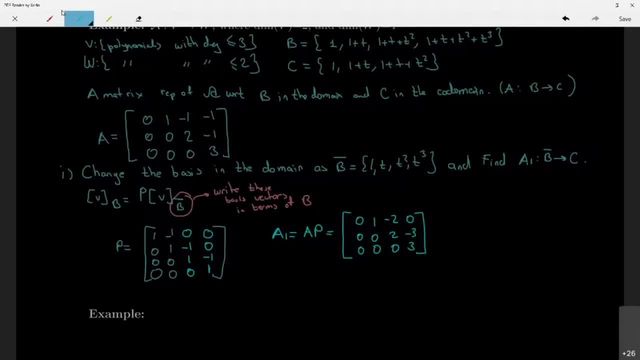 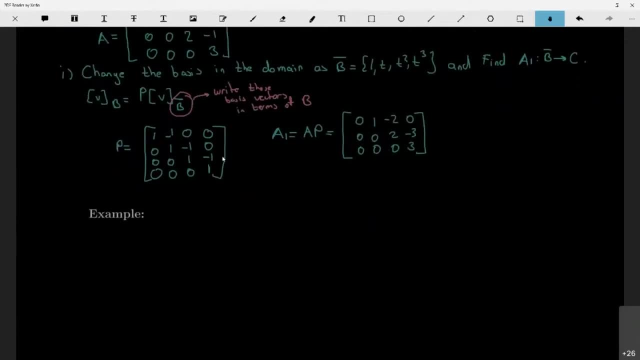 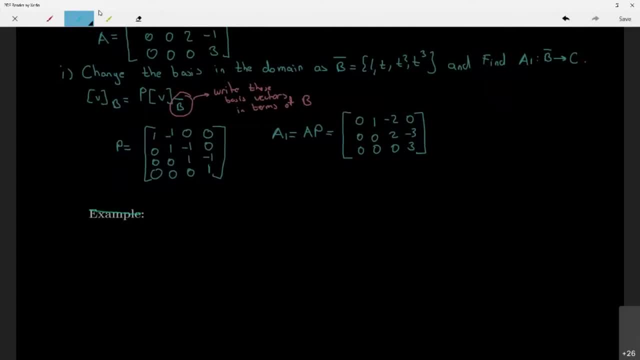 let's also change the basis in our codomain. okay, so say part two over here. so change the basis in the codomain s S C bar. okay, which is equal to: if I tell you the canonical bit, means met merit at first one, oh one T and t square, which is also the canonical basis. okay, the canonical. 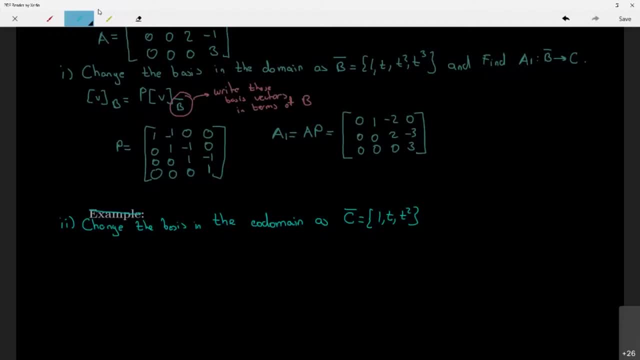 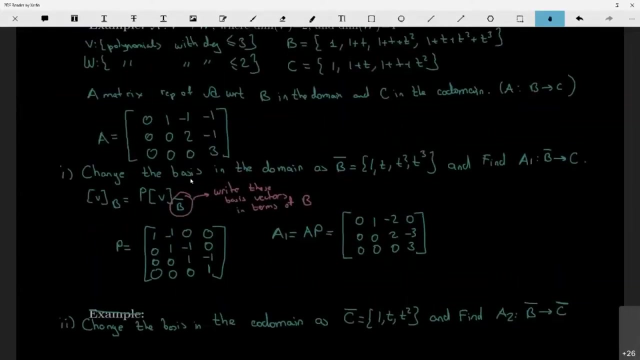 basis is the one with the one T and T square And find, let's say, A2, which is from B bar to C bar. So notice that the A matrix was given for B to C. So this A matrix was given for B to C. We found A1 for B bar to C bar by changing the base in the domain. Now we 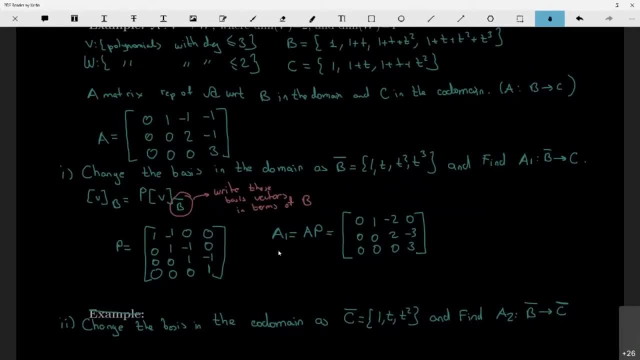 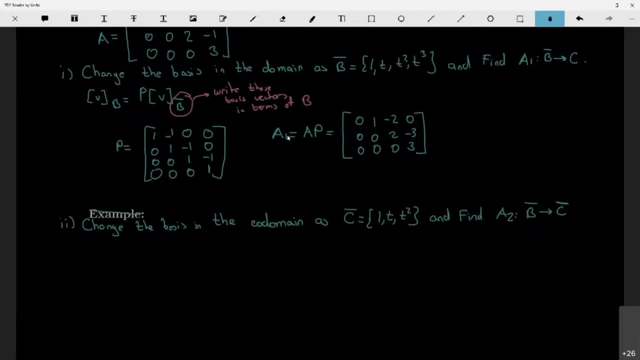 want to change the base in the codomain as well, So what I should do is that I should get this A1 matrix And multiply by a Q matrix, right, So I decided. so that is Q A, P. A bar is going to be equal. 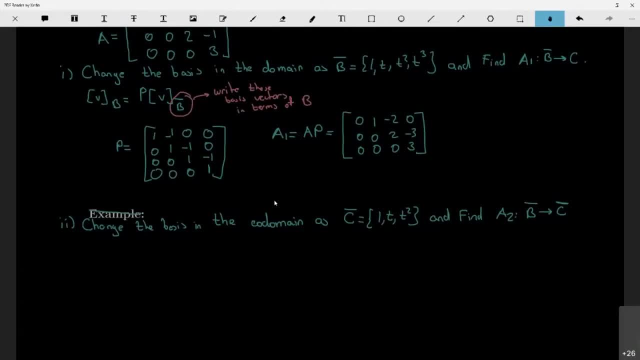 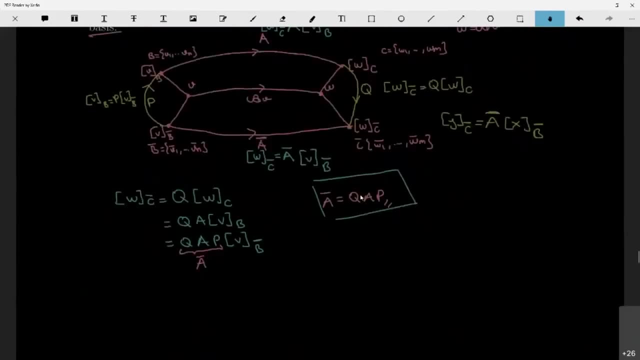 to Q A, P. And what is that Q matrix? So let's go up there. Okay, so this was what we are relying on. So this Q matrix takes the representation of any vector in the codomain with respect to base of C and transforms that into its representation with respect to C. 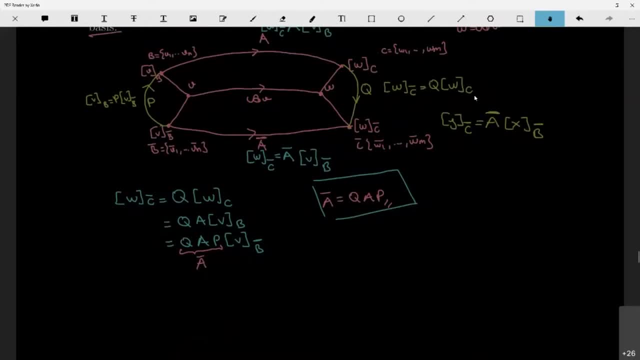 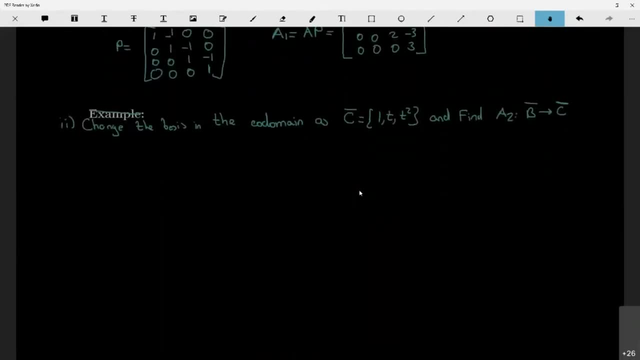 bar By multiplication. okay, So I'm looking at Q matrix over here, So let's do that. So I will go down, okay, And I would like to write that Q matrix, okay, such that representation of W with respect to C bar is equal to Q times. 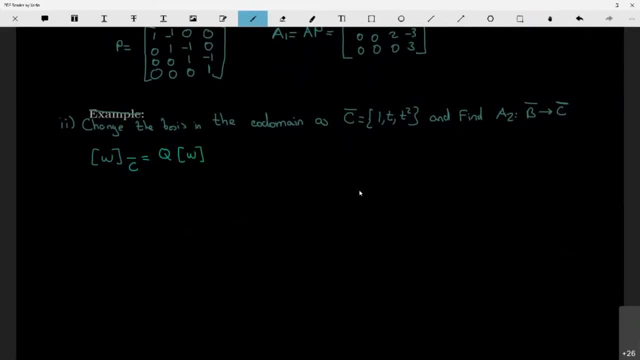 Okay, And how do I do that? I write down the vectors in C. okay, in terms of the vectors in C bar. So let's do that, So then you can tell me what the Q matrix is. okay, So Q matrix. 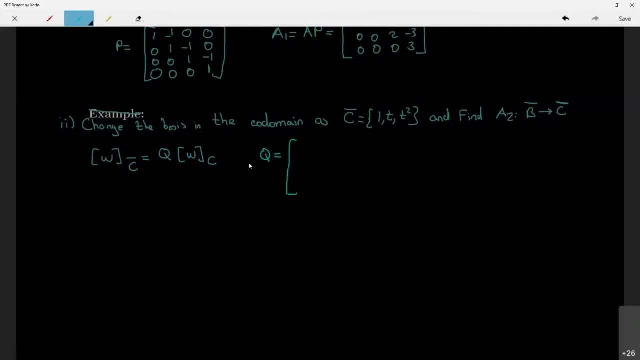 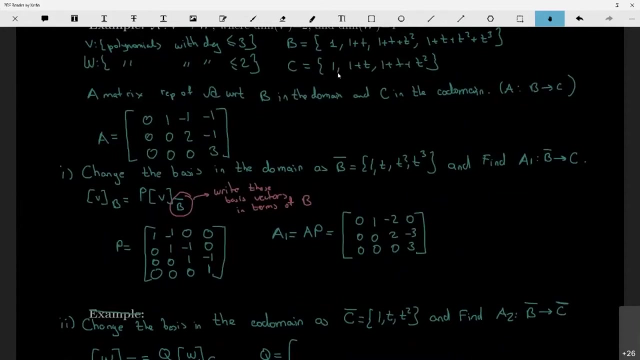 is that? So I should be able to write the vectors in C in terms of C bar. So what are the vectors in C? So let's go up and check. So now they look C. Okay, so C is 1, 1 plus. 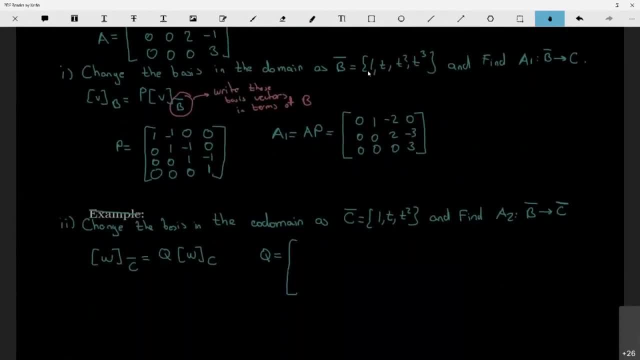 T, 1 plus T plus T. squared, so it is easy. So how can you express the first term, 1, in terms of these guys, It is 1, 0, 0.. And the other one is 1 plus T. in terms of those. 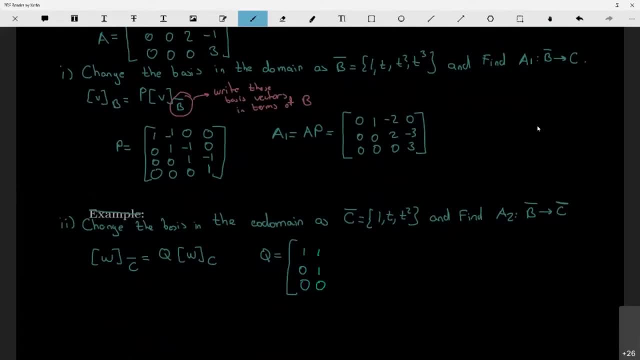 guys, is 1.. 1, 1, 0.. And 1 plus t plus t square is equal to 1, 1, 1.. Okay, And as I said before, so a2 is simply equal to q times a1.. Okay, And that is equal to, if you get this q matrix. 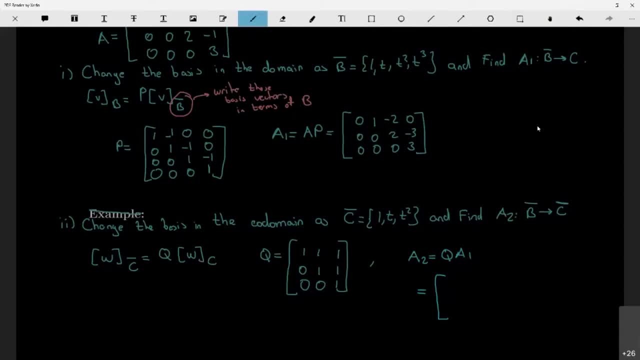 and multiply by a1 over here maybe I should also write this: it's also equal to q times 8 times p, And that is equal to 0, 0, 0, 1, 0, 0, 0, 2, 0, 0, 0, 3.. So we found the matrix. 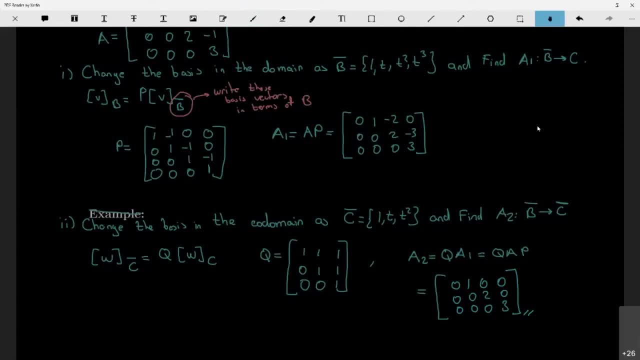 such that so any vector, if let's say v, w is av, and representation of w with respect to c bar is equal to a2 times representation of v with respect to b bar, And also we found a1 over here. So